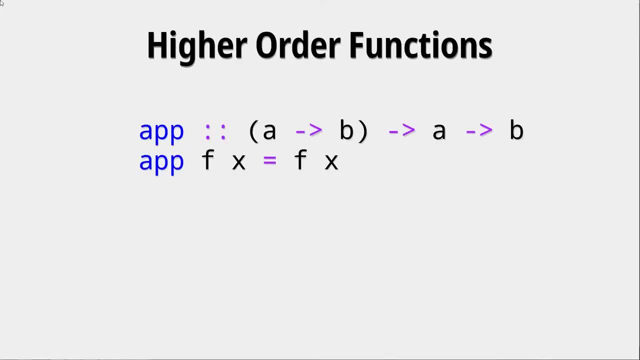 In this video we are going to look at higher order functions. A higher order function is a function that takes a function as an argument. So here, for example, we can see that this app function takes an argument f and that has to be a function because it is applied to x in its definition. We see this in the type signature. 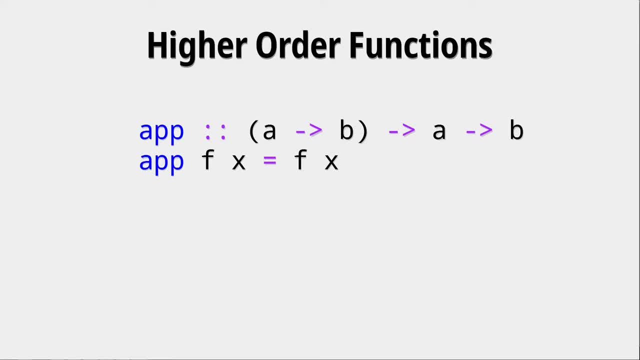 with the parentheses. The first argument is a function that takes an a and gives back a b. Let's look at an example with this: add one function, where we have a function that adds one to a certain number, and here we can see how app applies this: add one function to one in order to. 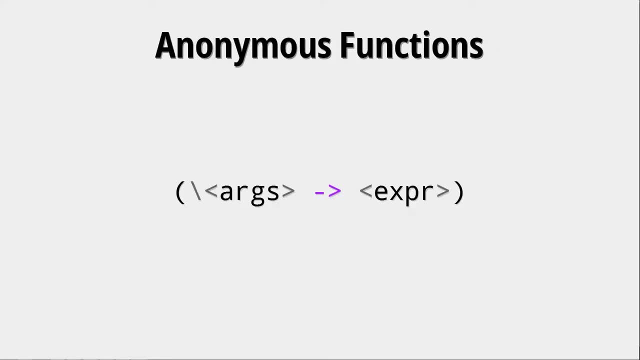 get the result. two: An important part of of higher order functions are anonymous functions, because we do not want to define functions with a name all the time when using them in this higher order function context, which is why anonymous function makes a lot of sense. So an anonymous function is: 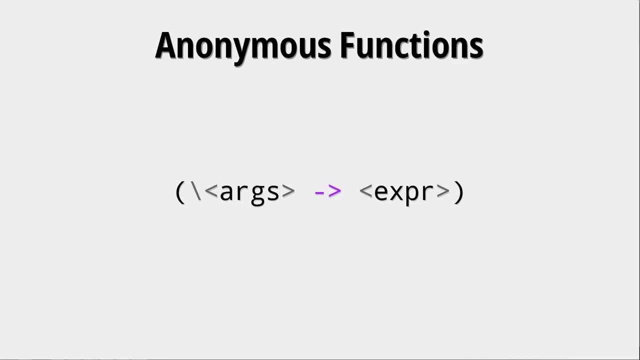 a function that does not have a name. when defining the function, It consists of a backslash and a list of arguments and then an expression. This is very similar to how lambda calculates the number of arguments and then an expression. So here is a very simple example. This would 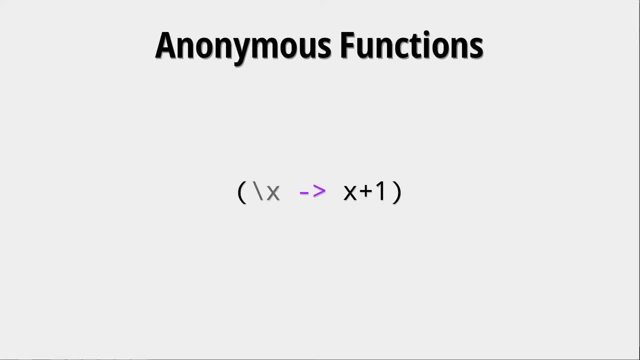 be a function that takes one argument, which is called x, and increments it. So what we could do is we can save the definition of this anonymous function in this variable we call add one. It is very important to see that functions are just values in Haskell. 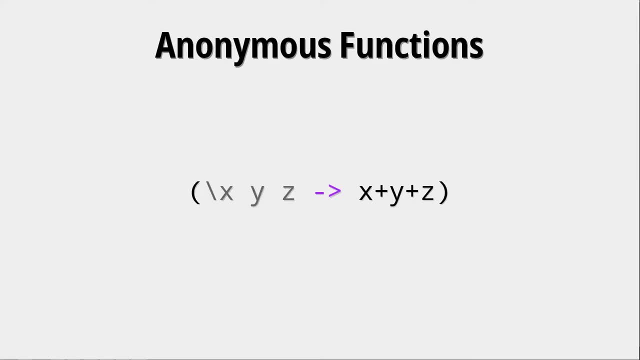 That is why they can be given as an argument. Of course, if you have multiple arguments, you do not have to write any commas. Commas would be a mistake here. Just write the argument list like you would in a normal function. Okay, and here we can see the application of anonymous. 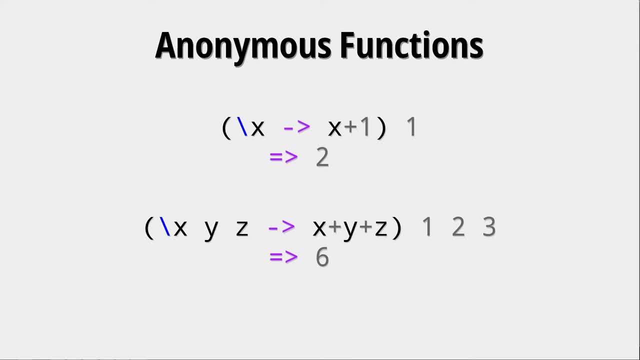 functions. This would also work within your code. So here, for example, in the first example, we apply this unary function that just increments a number to one, And in the second example we have multiple arguments. Okay, so here we see the example where we do not define this. add one function explicitly, but 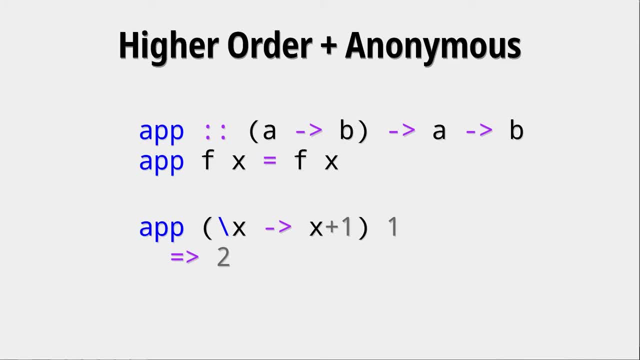 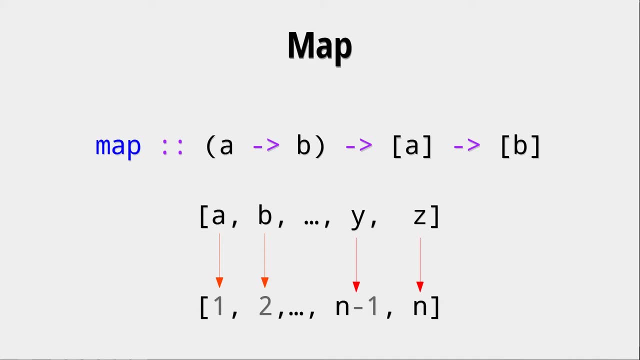 we just use an anonymous function in order to get the same result. Okay, so let's look at two very functions that are higher order functions and that are used often in day-to-day Haskell programming. The first is map, which maps one list of this type. 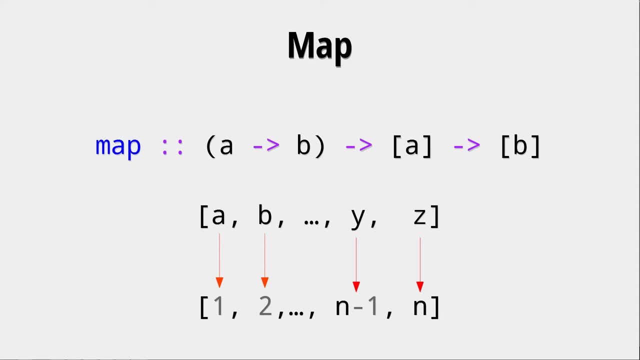 A to another list of this type B, and it uses the first argument, which is a function. it uses that in order to convert one list into the other. It's important to see here that the type of the list can very well change. The first list has the type A and the second list has the type B. Okay, so here's a very 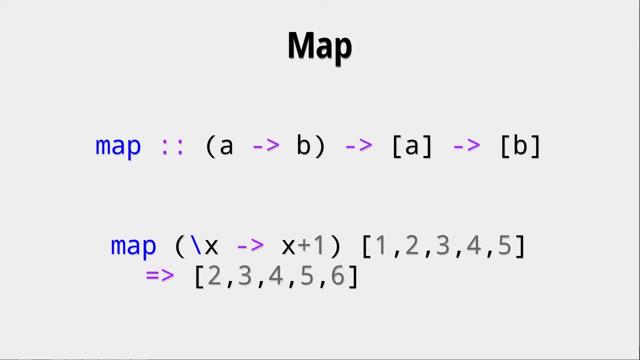 easy example with an anonymous function that simply increments every single number within a list. And here's another function. in one of the earlier videos we looked at a list comprehension that took a list of tuples and converted them to a list of the sum of the tuples. 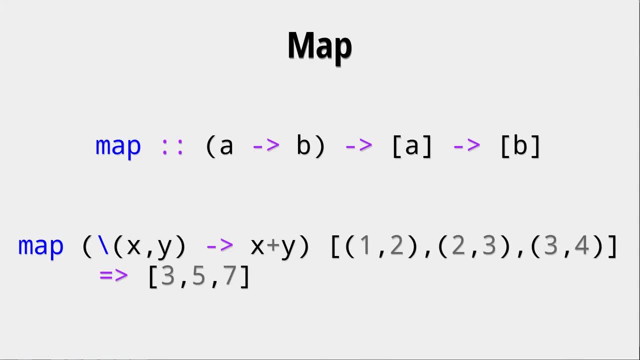 This map function does the same thing. We can also see that doing this pattern matching on tuples works within an anonymous function. So that's what map could be used for. Another very important function is the filter function. This one takes a function as its first argument, which always gives you a bool. 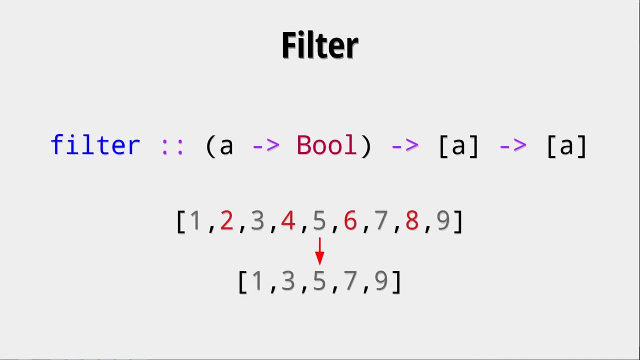 and this is what we call a predicate. This function is a predicate because it tells us whether, for a certain element within that list, a certain property holds, whatever that might be. Of course, the type of the list is not changed. We get an list of type A and we return a list of type A. So here, for example, we